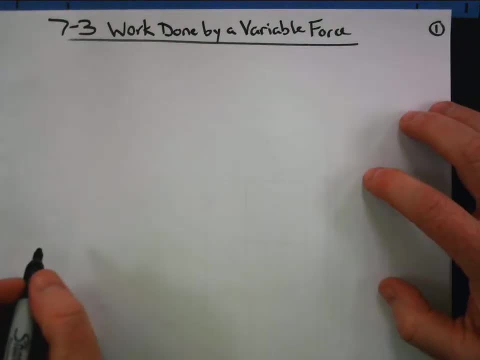 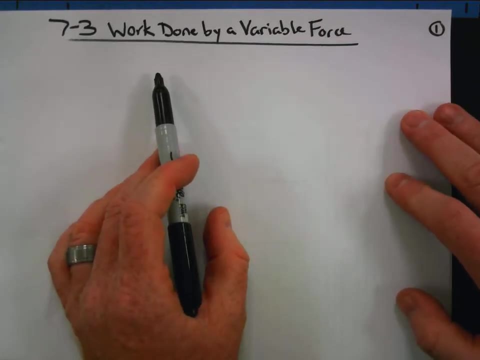 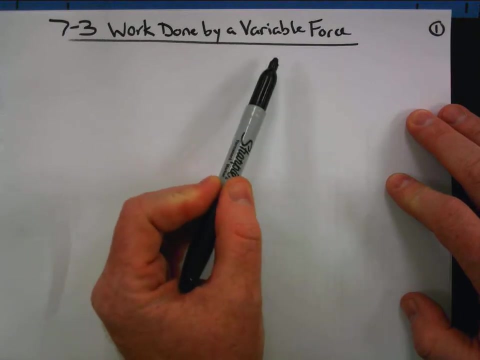 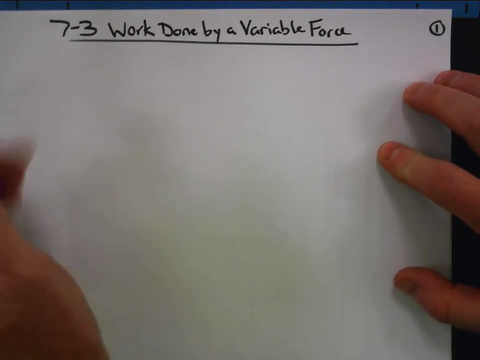 Hey guys, welcome back. This time around, we're going to be talking about, obviously, work done by a variable force, And what that means is work done by a force that's acting on an object, but the amount of force changes. It's not a constant value- And so it's going to have some specific applications for us. 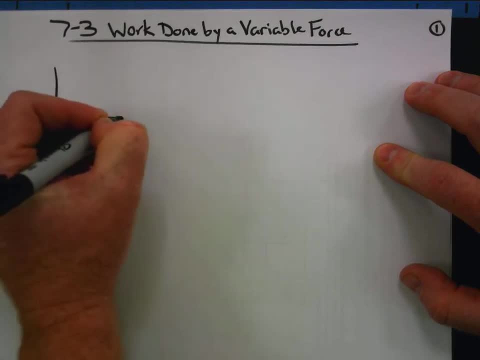 First, I want to look back, though, and just remind you of a couple things. If you're going to look at motion of an object, you can look at a position time graph, And let's say the position is changing. Well, that's good. That means the object is moving. 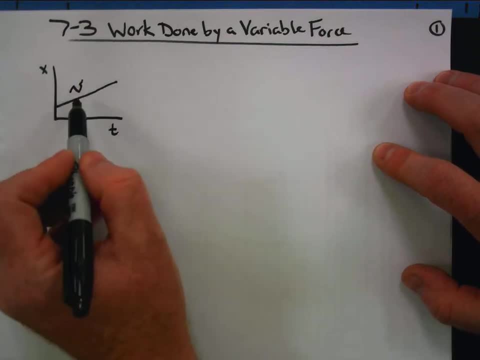 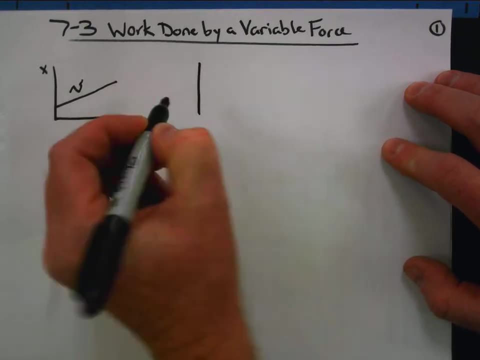 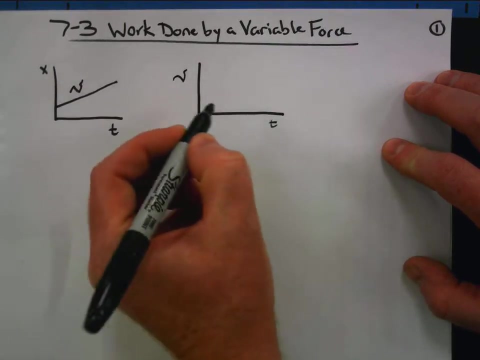 If it's moving, it has a certain velocity And the slope of this line represents that velocity: displacement divided by time. You can also look at the motion of an object whose velocity is changing And you would look at a velocity time graph in many cases for that. 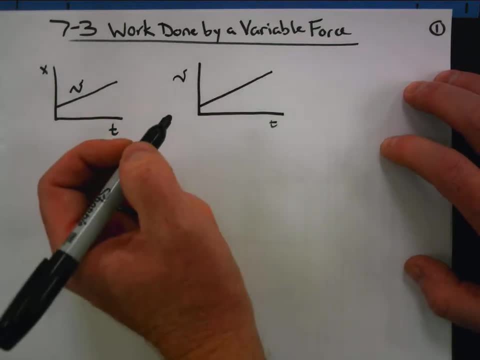 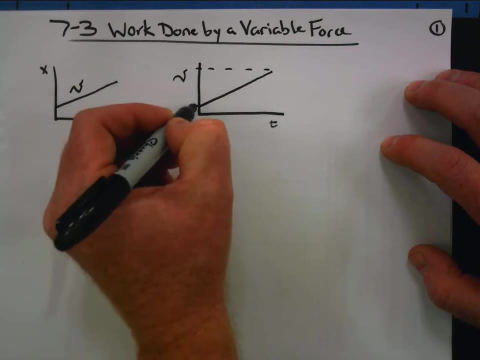 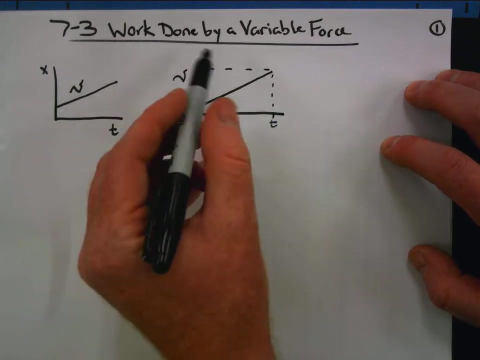 And let's say the velocity is doing something like this: Okay, Well, what we see here is a change in velocity from this value to this value over a certain time interval, from there to there, And the amount of change of velocity divided by that time gives us the slope of this line. 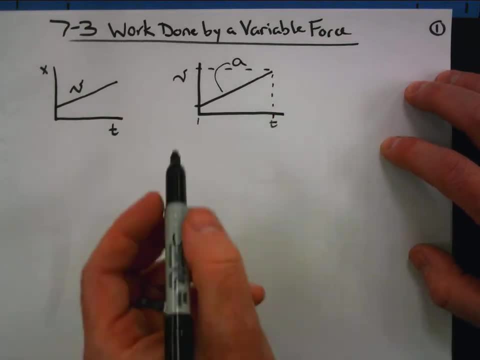 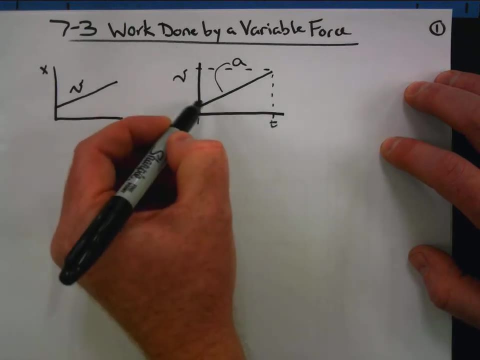 And the slope represents the rate of acceleration of the object. But there's more hidden in here. As the object is moving, or as its velocity, As the object is changing, it is moving, So it's covering a certain distance, And that distance is seen here in the area under that graph. 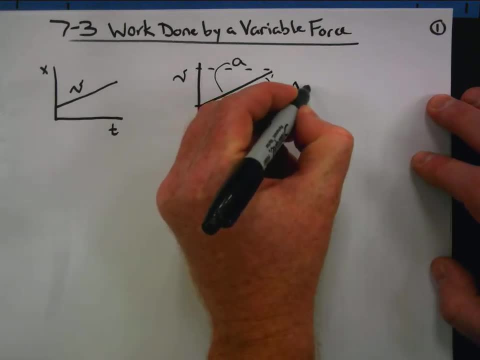 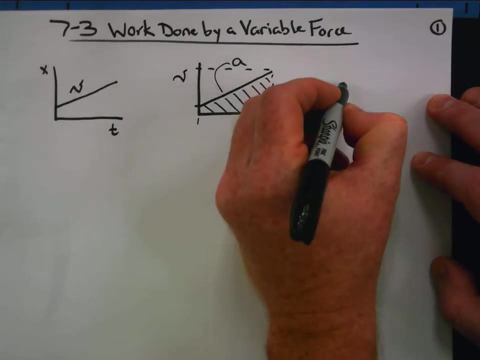 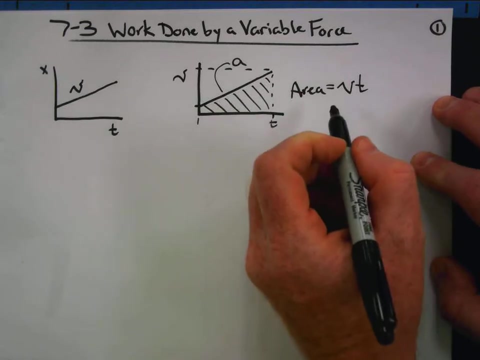 When we look at this area, we can say, well, we're looking at this dimension of velocity and this dimension of time And we multiply those together to find an area In some way. You know, it's not as simple as this when this line has a slope to it like this: 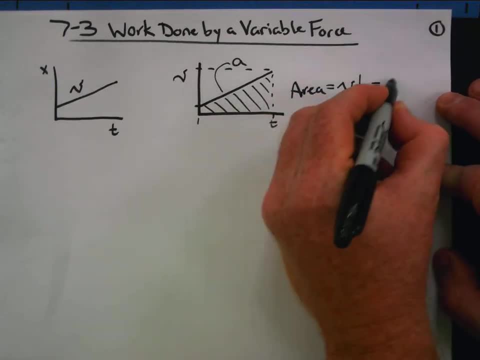 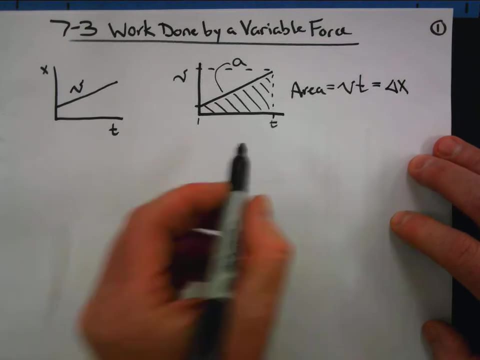 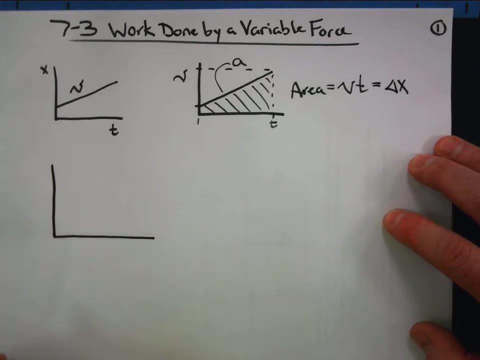 But you get the idea: Velocity times- time is going to give you a displacement or a change in your position, And that's what we're doing. So now we're going to look at the same way of viewing something that's happening, But we're going to look at different quantities. 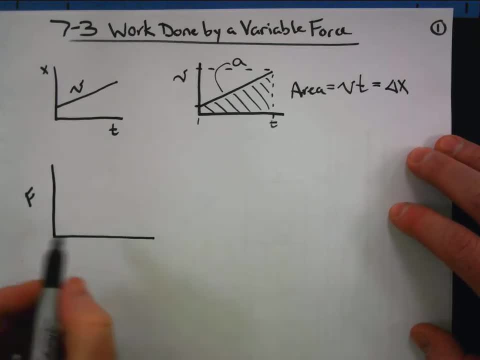 We're going to look at a force that is applied to an object, And that force is applied while the object moves a given distance. At first, we started looking at forces that were constant, And so on this graph the slope is zero. 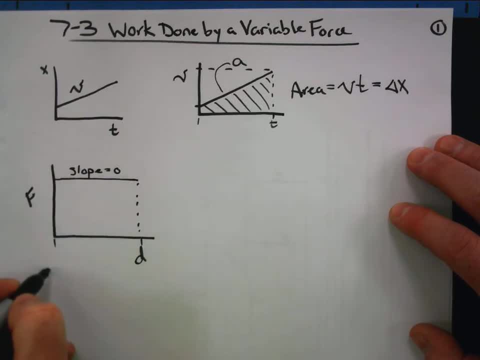 And if we wanted to find the work done by that force well, we would take the force, multiply it by the distance That would give us the area under this curve or under that line. force times distance: Okay, fine, Not a problem. 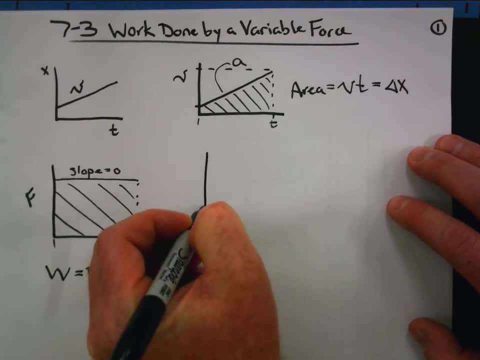 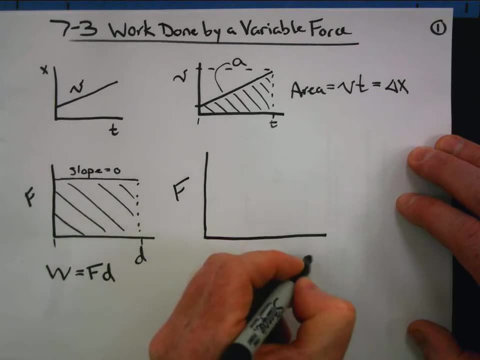 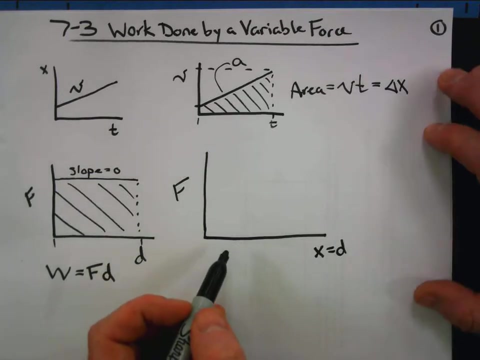 But if the force is a variable force, then things change a little bit, So we have a different force. I was about to write x, so there we go. Well, x is just d for distance. That's fine. Now, if the force is a variable force, we might see something like this: 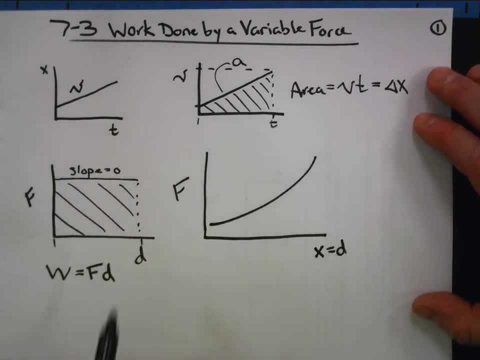 As the object moves, a force is changing, And this one's kind of extreme. If we wanted the work done by this force, we would have to look at the area under this curve, And without calculus, we don't know. We don't know. 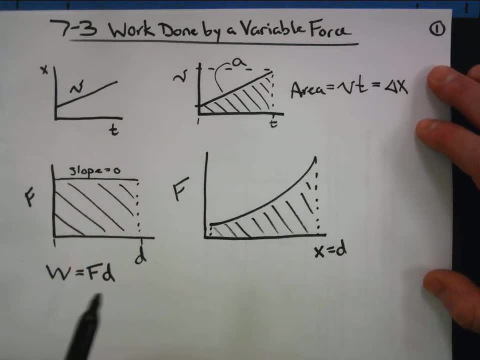 We don't have much of a chance of doing that. Not really It could be approximated, but that would be about the best we could do. There is some way- I mean we're still multiplying this force, dimension with this distance dimension, to find that area. 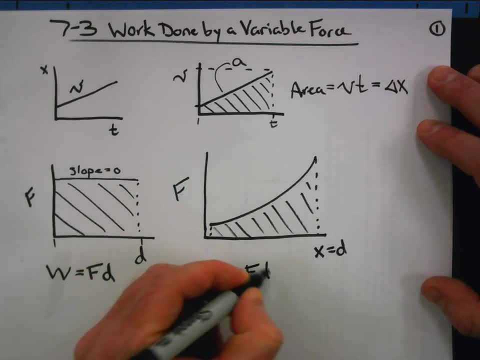 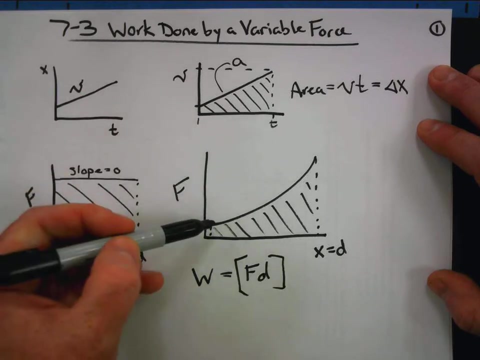 But it's obviously going to be more complicated than just force times, distance. But there is something here where that is happening inside And that will lead to the work done by the variable force. Fair enough, Thankfully we actually won't. We'll be looking at situations where the rate of change of the force is different. 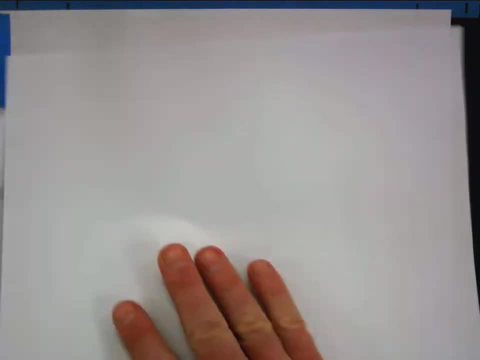 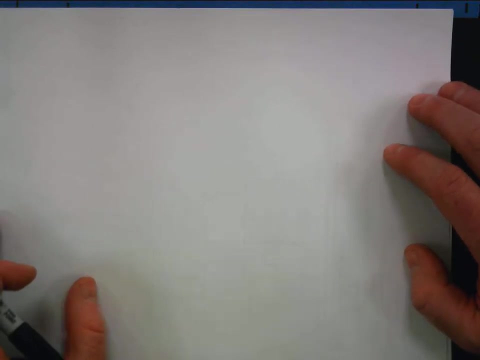 We're going to be able to look at situations that are a little simpler than that, And so let's take a look at how that might be viewed. We are going to have a force distance graph And we could say: well, you know, we're going to have a force distance graph. 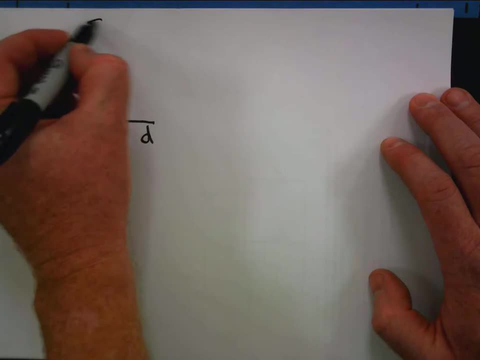 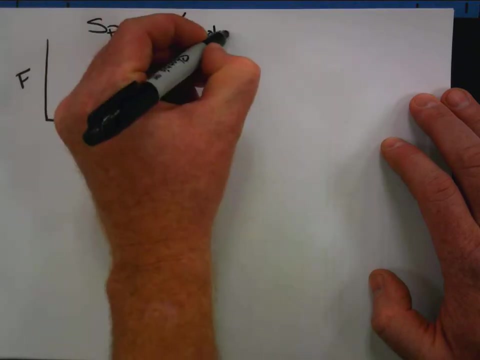 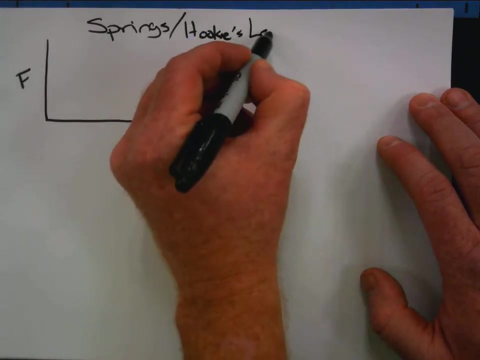 Well, you know what? What if it's something like a spring, And this is kind of neat. You know that springs obey Hooke's Law. quite often It's worth noting. not all the time, Excuse me, But quite often this is a very helpful thing we can look at. 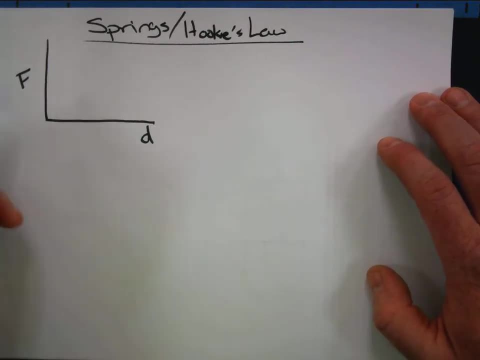 And what ends up happening is, if we have a spring that's already at its resting length, it has not been stretched at all. Well, there's zero force that I have to use. What do I have to use to keep it there? Fine, 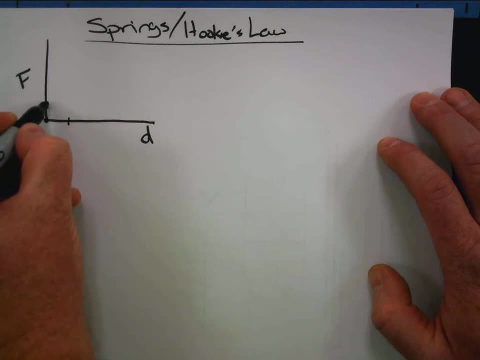 And then let's say I stretch a spring a certain distance, The force that is required to keep it at that new distance might be here. And if I stretch it to double that distance, double the stretch amount, a spring that obeys Hooke's Law would require a force about that large. 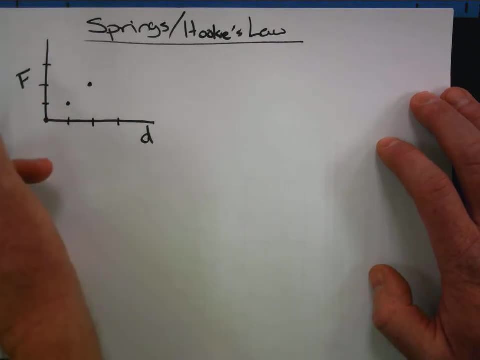 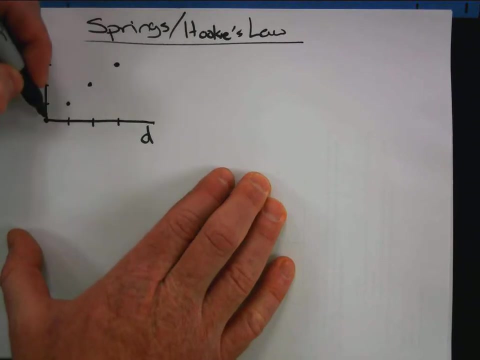 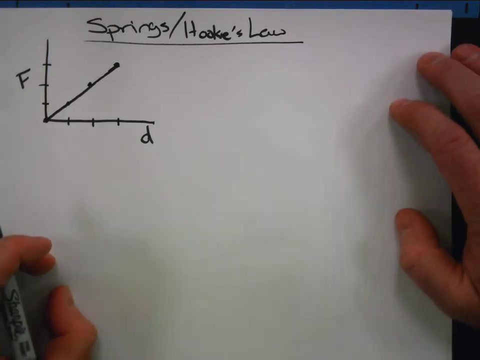 If I triple that stretch, then what I have is a force that is about there, And so we see a pretty nice linear relationship with springs that obey Hooke's Law, And you'll hear the term a linear spring. You may have even heard me say that before. 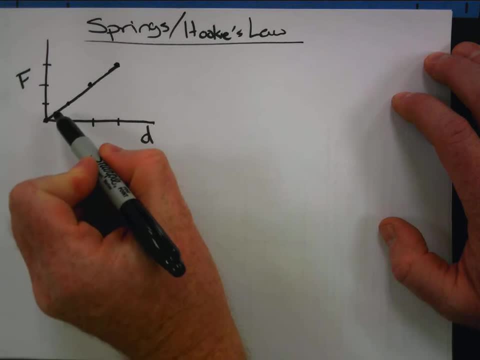 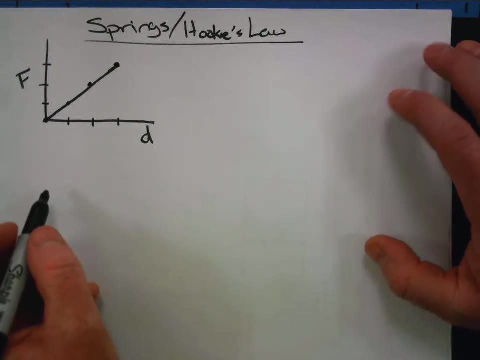 All that implies is that the spring is obeying Hooke's Law. We have this between force and distance, a linear relationship going on. But we know that force times distance equals work done. So we're going to take the force dimension, multiply it by the distance dimension here. 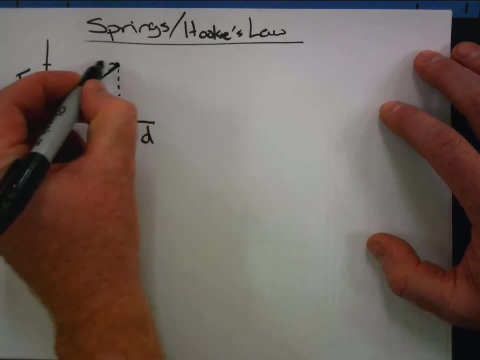 But what we need to keep in mind, of course, is that if we just do this, force times this distance, we get the area of the whole rectangle, And that's not what we want. We just want the area under the line, So to find the work done by this force. 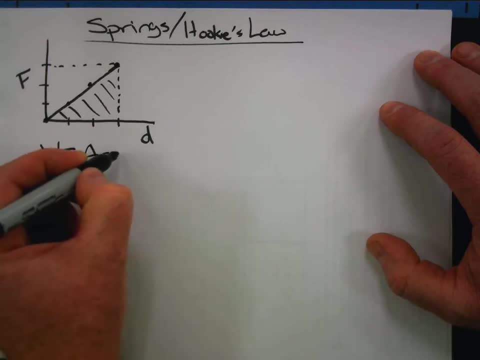 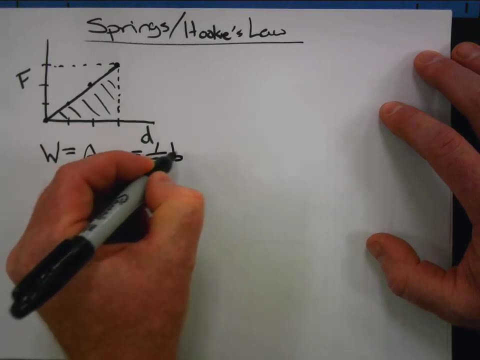 well, we know we want to look at the area And this shape happens to be a triangle. so the area is going to be represented by 1 half base times height And that's the area of a triangle. Okay, no issues there. 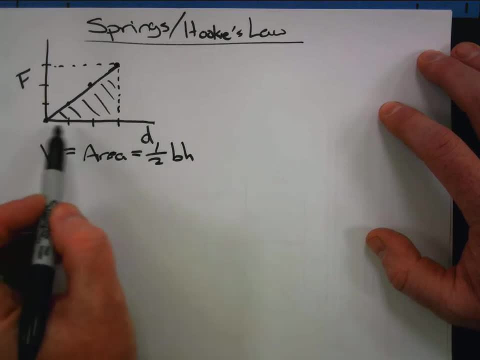 What is the base of the triangle? The base is just our distance d. So we're going to have 1 half and the base is distance d And the height. Well, the height, sure we're going to have force. 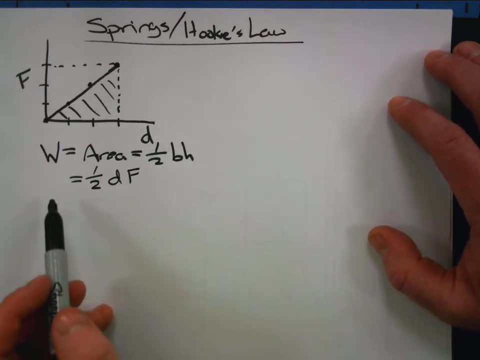 Okay, And it's interesting to note. well, if this is a constant linear relationship here, we might even be able to say: if we look at the average force, then it's going to be somewhere in the middle or half of the total force. 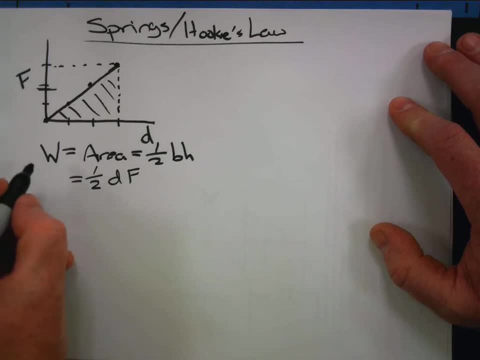 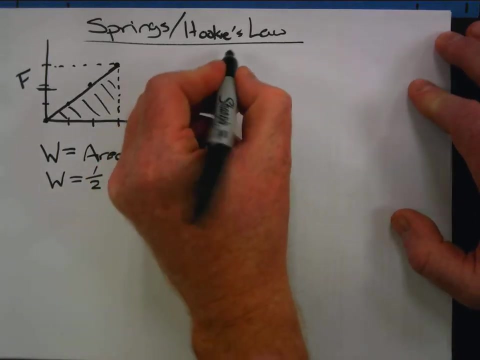 Never mind that for now. But when you read this section that idea of average force is going to come up. So if we're looking at the work done, this idea of 1 half force times this distance is expressed a little differently. Think back about Hooke's Law, Hooke's Law itself. 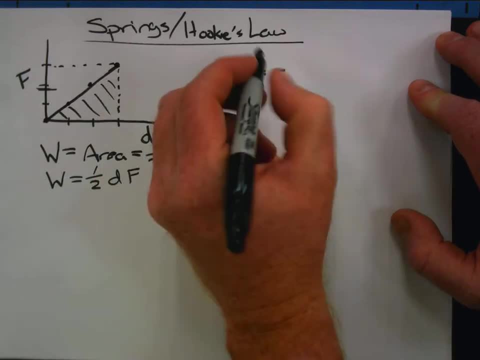 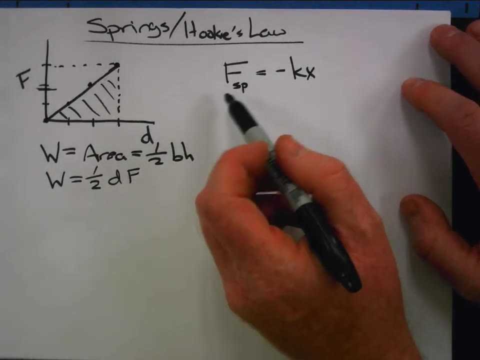 It's the force of a spring and it's equal to negative kx. And this is actually the restoring force: how hard the spring is pulling back or pushing back. k is your spring constant, x is the distance of stretch or the amount of stretch. 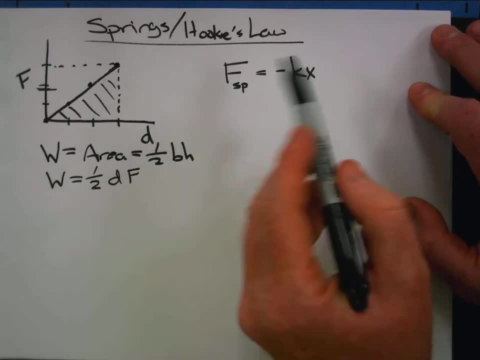 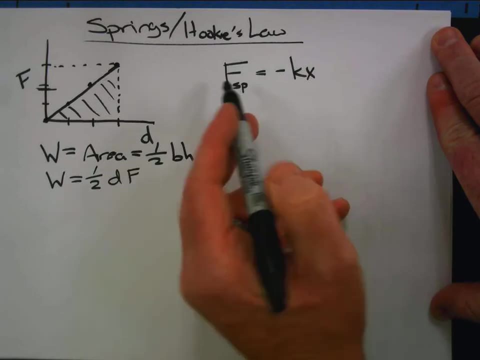 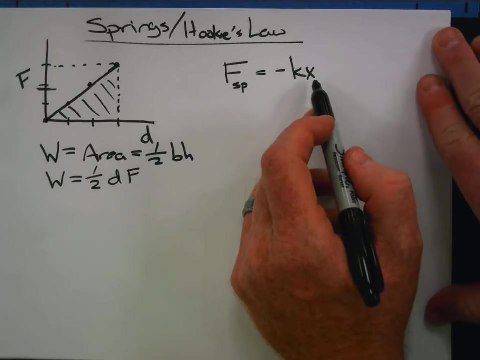 the amount of compression. possibly This works for both stretching and compressing a spring. The negative sign here is simply indicating that our force of the spring will be in the opposite direction as the stretch or as the compression. So if we stretch one way, 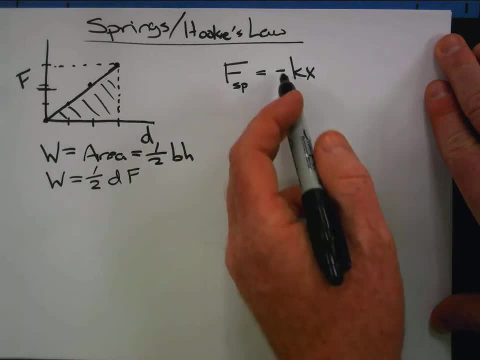 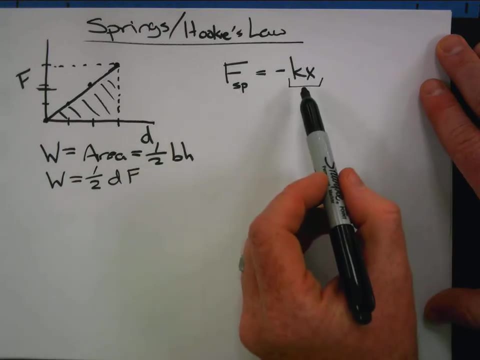 the spring wants to rebound the other way. That's all the minus sign is telling us. But what we have here, we don't need the minus sign at the moment. we have this And we could look at a substitution here. We could put kx in for this f. 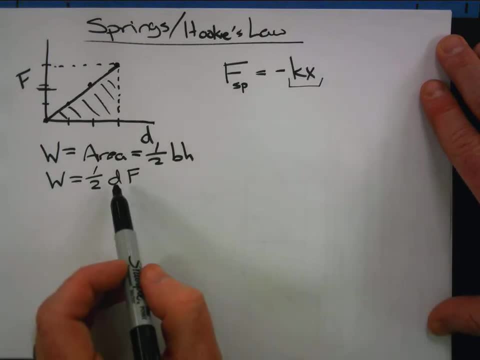 And since we're using x for a distance, I'll switch the d to an x all the way. Also, I could have done that in the beginning. It's just, you know, it's a little better to be consistent, possibly. 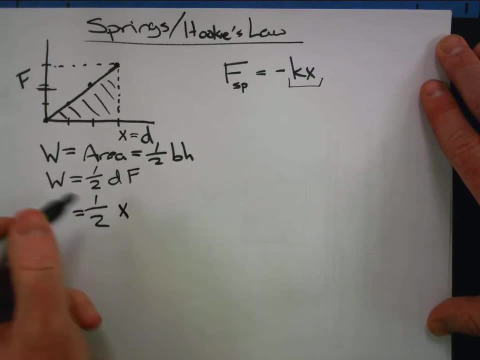 So this equation is going to become 1: half. My d is an x. right there There's the distance, And instead of force I'm going to write kx. Okay, So I'm still looking at the work done by this variable force. 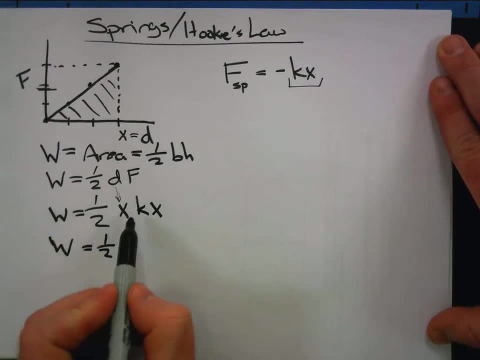 There is this 1 half in the equation, But look what's going on. I have k times x, k times x squared And that's going to be a handy equation to use. If you look at this, it almost seems similar to the equation. 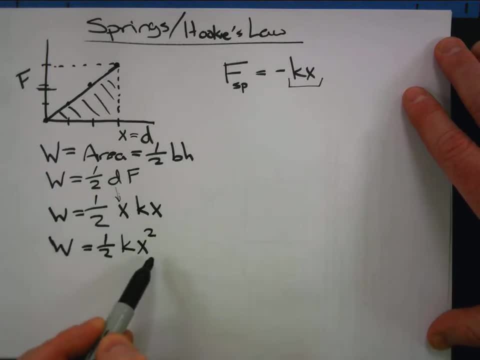 for kinetic energy: 1 half mv squared. Well, here this is the work done by a variable force: 1 half kx squared Now, k is still your spring constant. You would still have to know that information about the spring in order to find out. 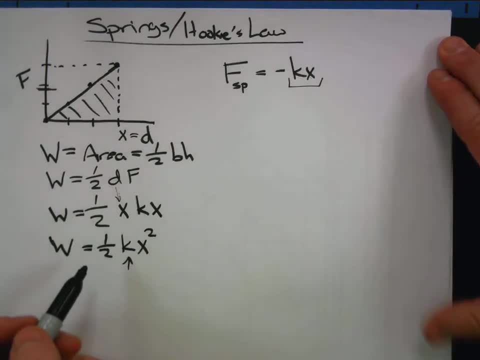 the amount of work done. But it certainly is possible. Or you might some other way come about the amount of work done and thereby be able to determine the spring constant. Like many of the problems, it can work either way. So next step, and this was page 2,, by the way- 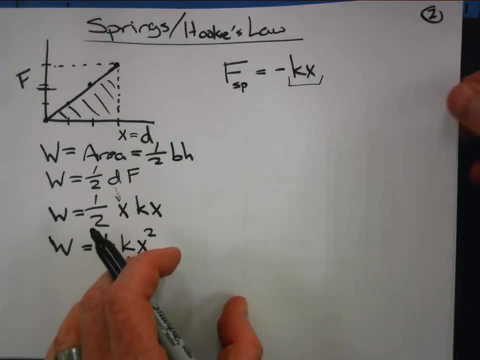 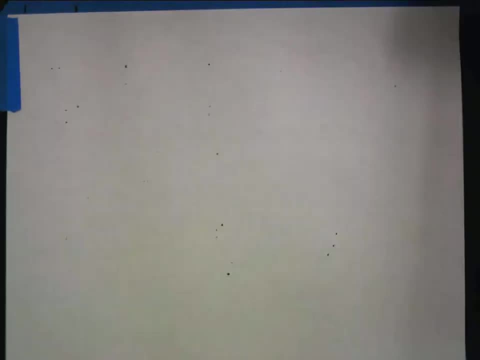 Next step. what I want to do is I want to show you an example of this. How would this actually look Like that all marked up? So, pardon, the bump on the camera. Sorry about that. I'm going to have this apparatus set up. 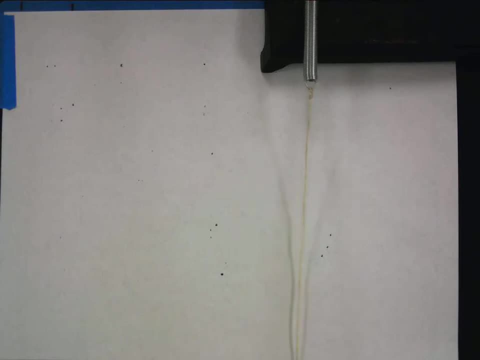 And this is simply a spring, And I have this string attached to the end of the spring And there's going to be a loop of string here And I will have a mass hanging from the spring or from the string. The string is actually going over a pulley. 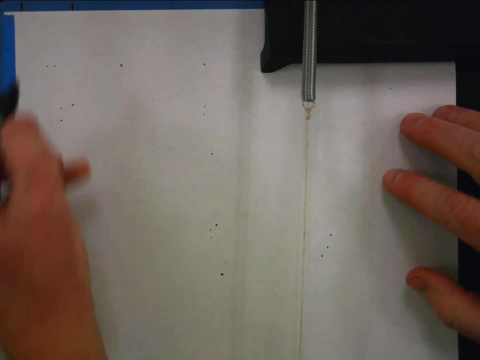 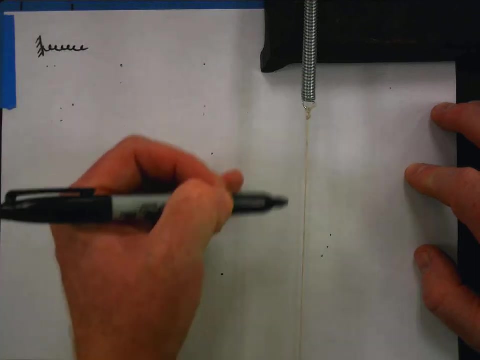 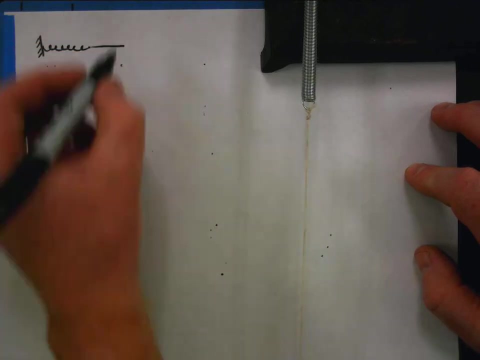 I'll give this a quick diagram So you know what I'm talking about here. The spring here that you're looking at is attached to some fixed structure. There's our coil spring. There's this string on the end of the spring. The string is being redirected around a pulley. 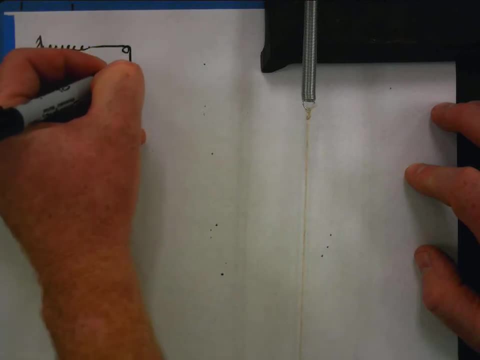 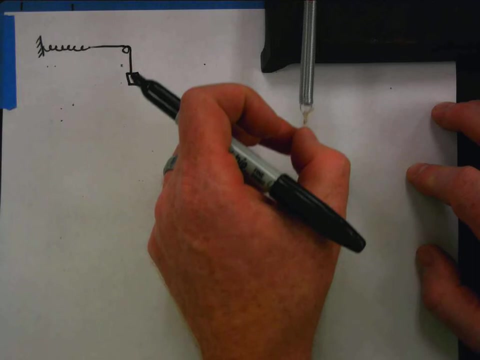 The pulley is off camera here, But it's allowing that- And then the mass is pulling down, creating the tension in the string which is elongating the spring just a little bit. You can see there's some ability to move there. 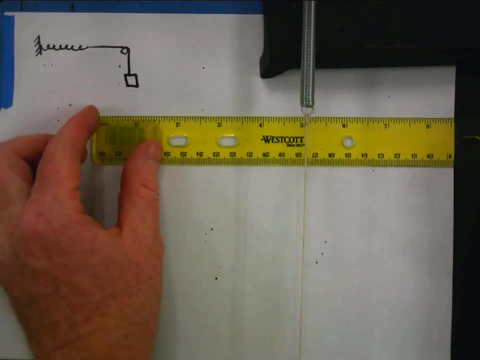 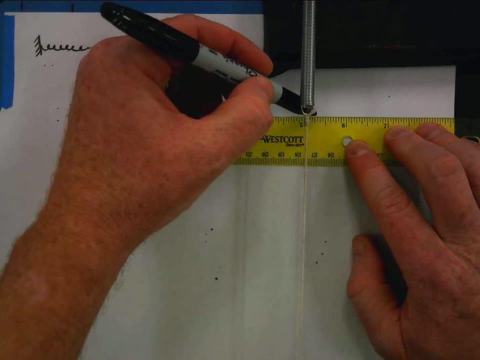 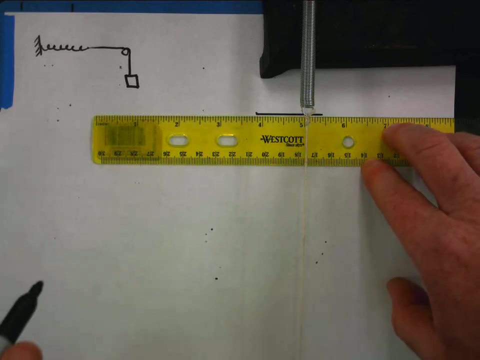 Okay, So we have this initial position of the spring. I'm going to mark that on the paper. And now to the camera's point of view. that mark may be off a little bit. I'm looking straight down And this part of the spring: 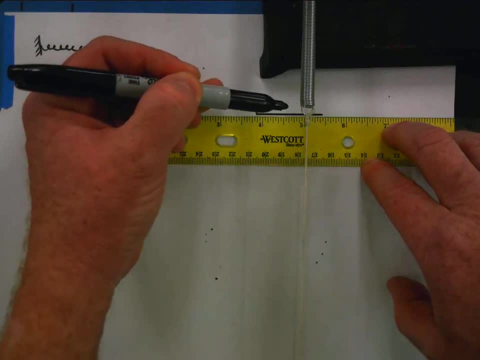 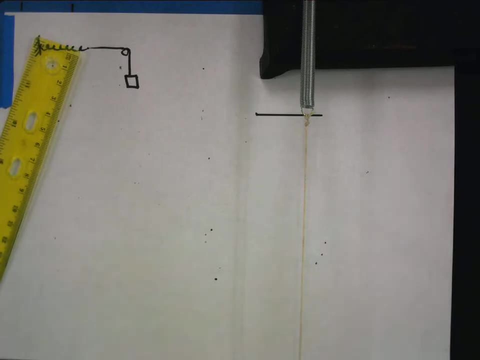 the last coil is directly above that line. So that's going to be how I will view this, And what I'm going to do now is I'm going to hang an extra mass on the spring so we get more stretch, more elongation. 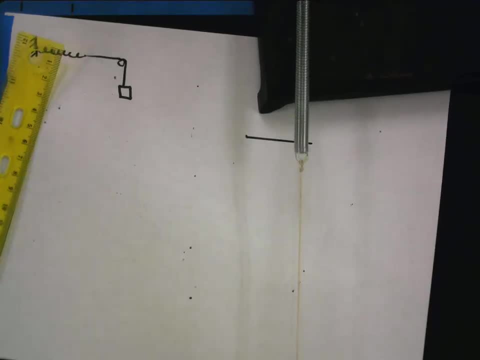 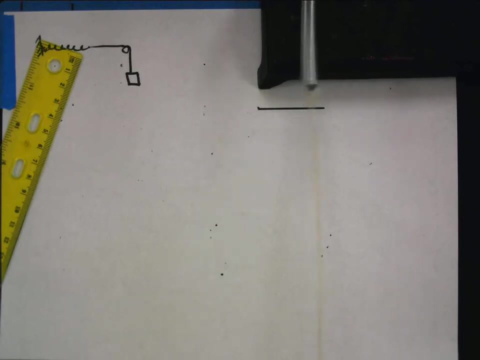 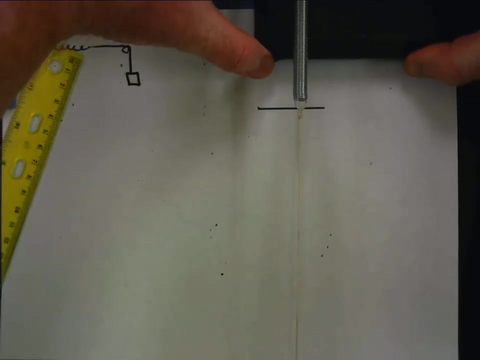 So, Oh, shoot, I forgot a part. Okay, I forgot that was going to move. Nothing to see here. Move along, carry on All those things So I can reposition this guy. You've got to forgive me. 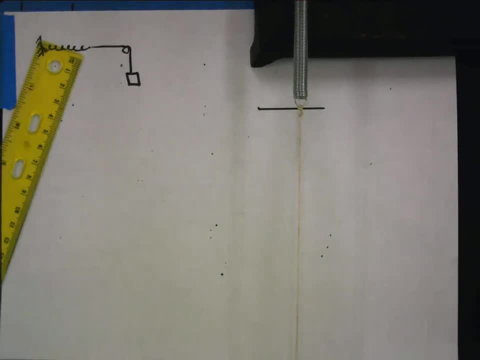 Bear with me A little error. Okay, I can lock this guy down, so it doesn't move, And I believe we are. We're good. We're good. Now, Pay attention once again As I Add more mass to the end of the string. 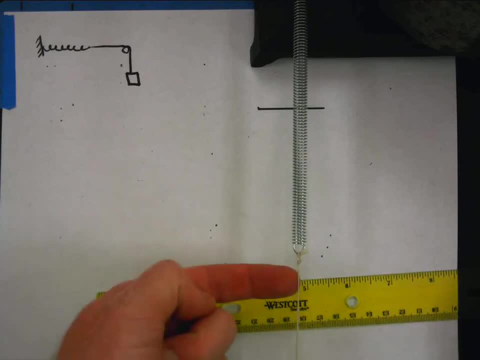 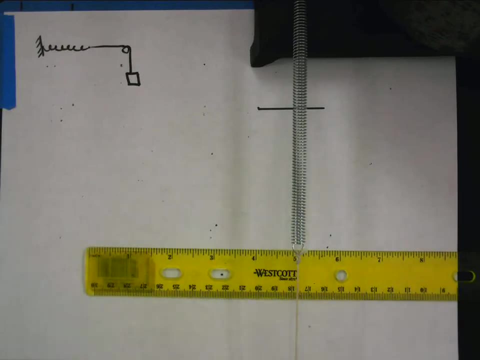 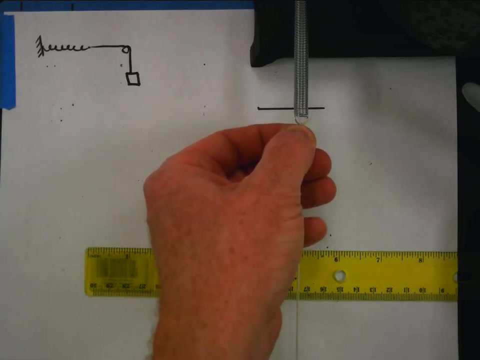 There's more tension in this string here. There's a larger force pulling on the spring, And so we have a new distance. Now the interesting thing here: To get from this position, there has to be a stronger pull, And the more it pulls. 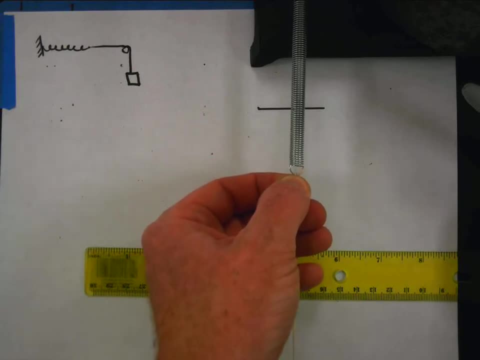 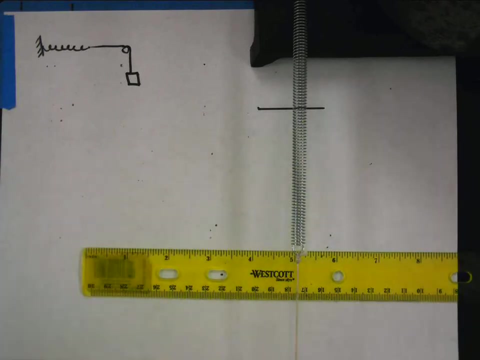 the more I have to- Oh, that's a terrible way of saying it. The further the end of the spring goes, the greater the force I have to use to continue to move it. So the force of pull is varying here. Variable force. 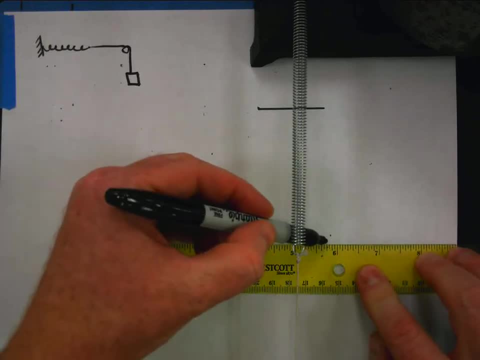 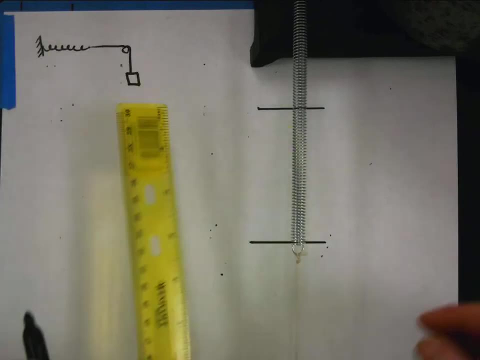 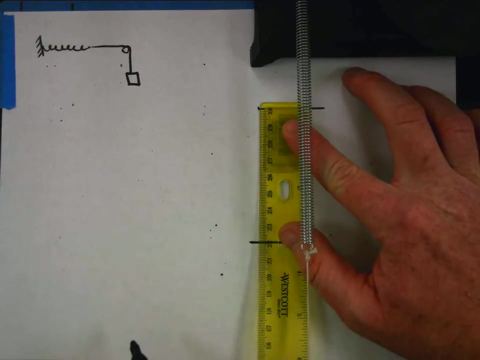 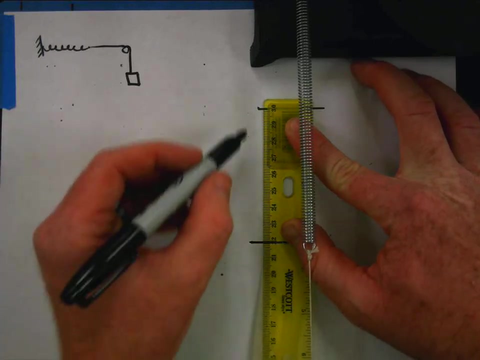 And I'm going to line this up again and get a mark for a new location. Okay, So what we've got is this displacement here. I'm trying to figure out where to put the ruler to get a good measurement. Okay, So, 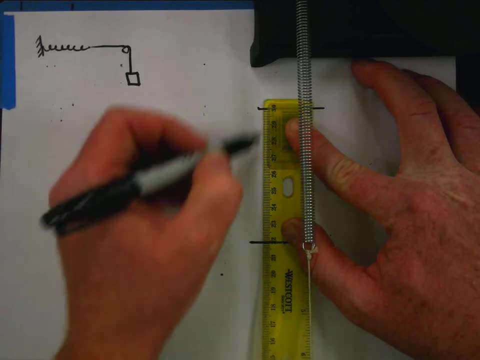 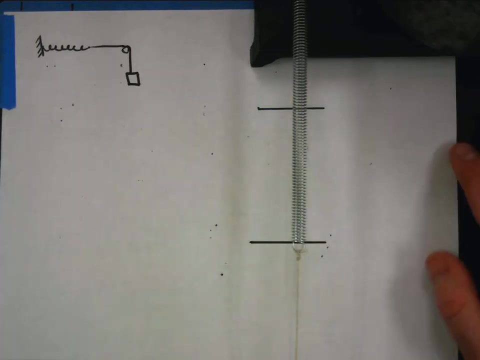 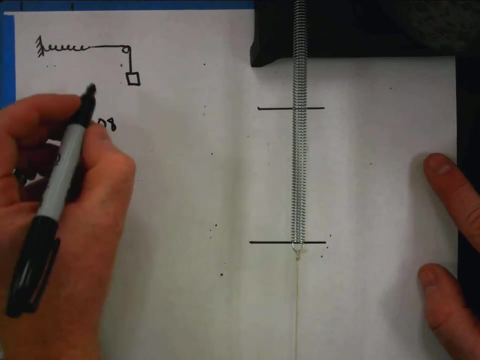 From roughly 22 centimeters up to 30.. Roughly, So that's a displacement of 8 centimeters. So I have this x value: 8 centimeters or .08 meters. All right, Well, what is the force I'm using here? 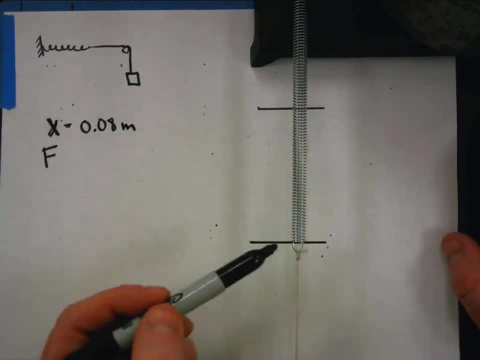 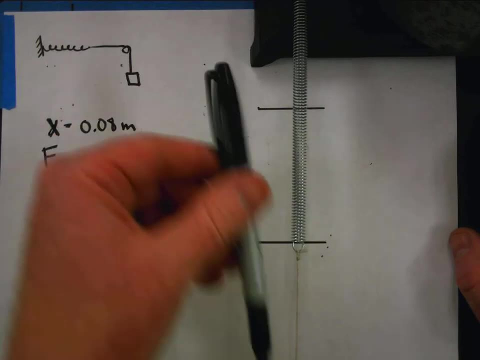 The amount of force that I'm using. Well, that's going to be At this moment. this end of the spring is in equilibrium, So there's a spring force back, but there's also this tension here. The tension here comes from a total of 700 grams. 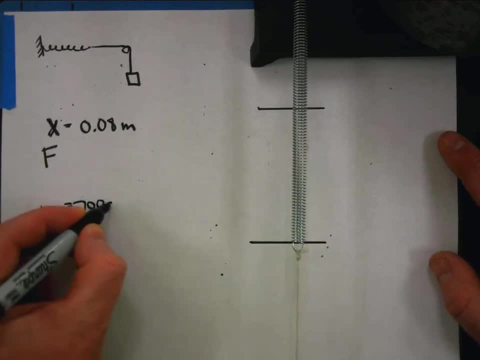 The mass on the end of the spring is 700 grams. The weight of that is mg And that happens to be the force that I'm using here. So if I know the displacement or distance traveled and I know the force, what is possible here? 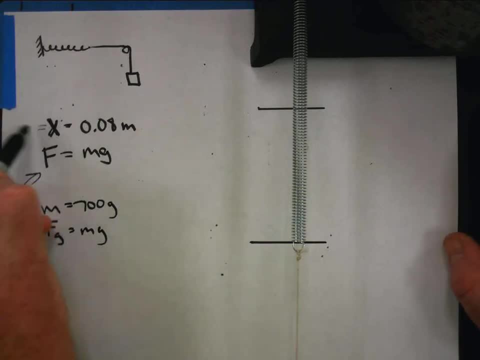 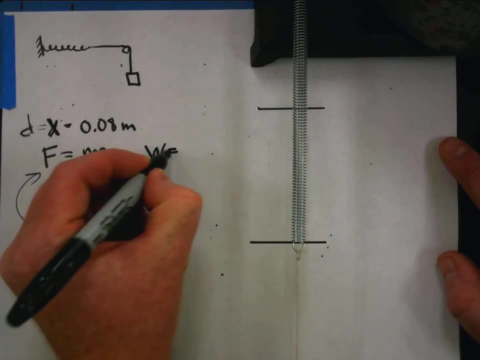 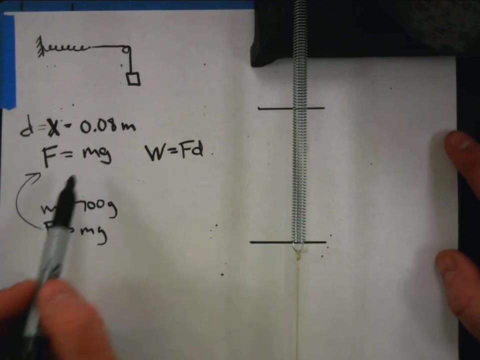 Well, I can find. This is my distance, Isn't it? This x is distance and I have force, And from force and distance I could find work. Or can I? This force, this mg is not the force that was applied. 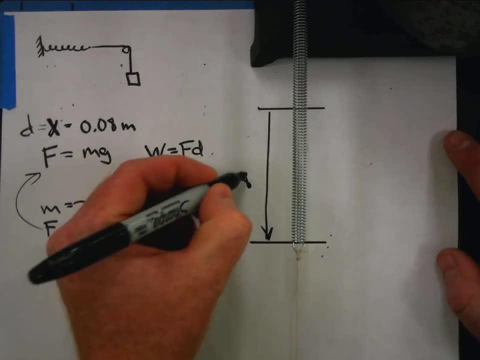 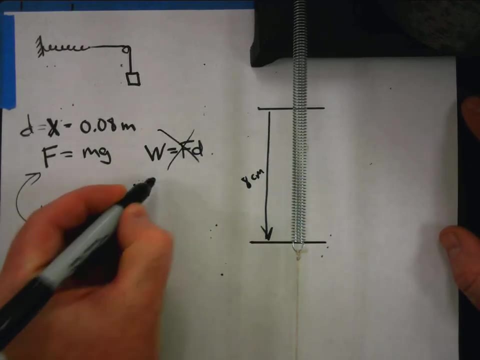 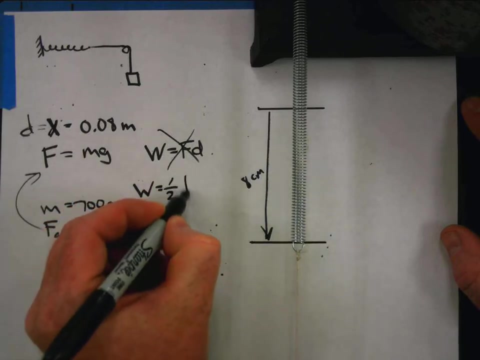 across that whole distance of 8 centimeters. So it's a variable force. So this won't work. What I have to do is look at the fact that this variable force can be calculated. It is related to the spring constant here and to the square of that distance traveled. 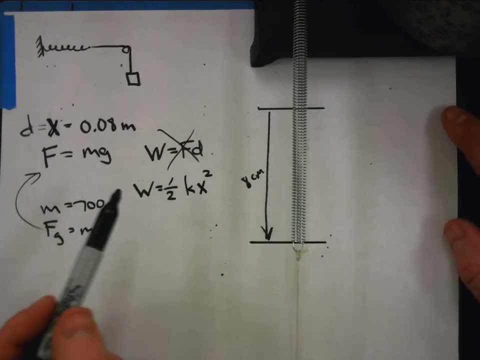 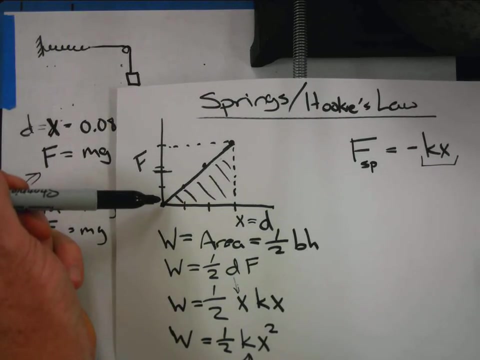 So the issue here at the moment is, if I wanted the amount of work done, I would need to know the spring constant, Or I might have another way. But that other way it goes back to this issue, this idea, since the force varied. 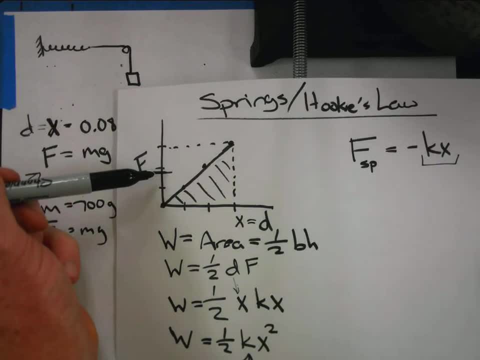 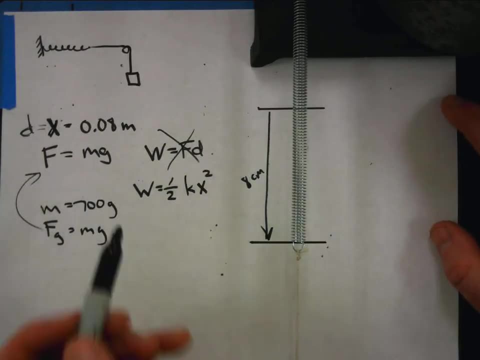 from one value to another. I could take the average force. Well, that's a little more work that I need to worry about at the moment, But you can clearly see that we have this new relationship where we can use this value, this arrangement. 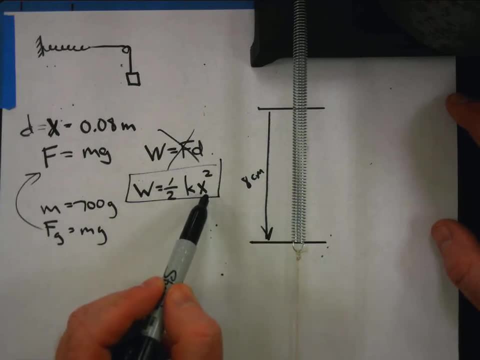 spring, constant amount of stretch or compression and use those two in this way to find the amount of work done. Keep in mind that other relationships may be tied to this, For example, if a spring is going to be used to launch something.